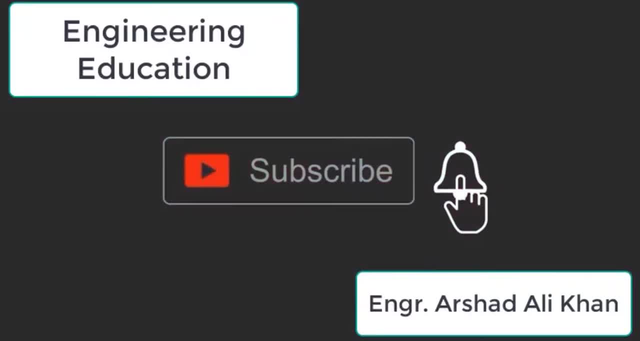 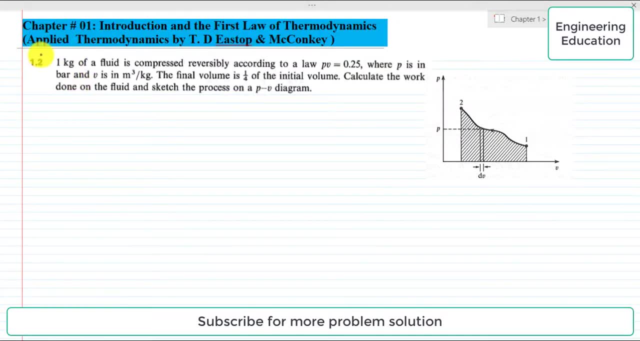 Hello students, welcome to my channel, Engineering Education. Please subscribe to my channel, Thank you. In this lecture we are going to solve problem 1.2, chapter 1, introduction in the first law of thermodynamics from the book Applied Thermodynamics by TDS Staub and McConkie. 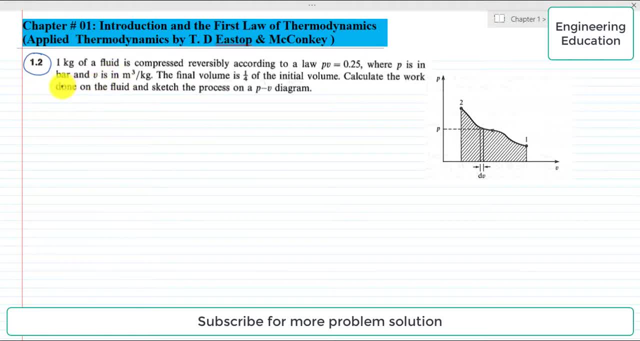 The statement of the problem is: 1 kilogram of a fluid is compressed reversibly. according to La, pv is equal to 0.25, where p is in bar, p is the pressure and v specific volume is in cubic meter per kilogram. The final volume is 1 by 4 of the initial volume. 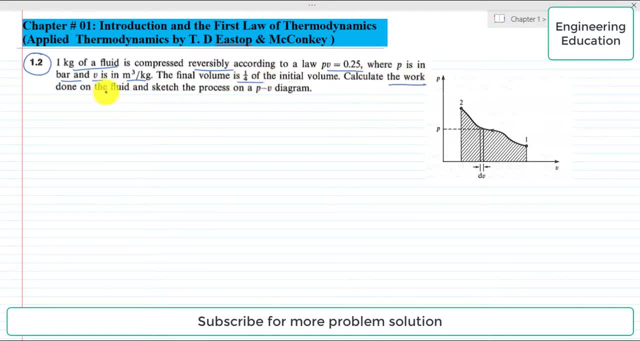 Calculate the work done on the fluid and sketch the process on p-v diagram. So first of all we will write the given data. So we have, given that the mass of the fluid represented by m, that is 1 kilogram, The law of compression. 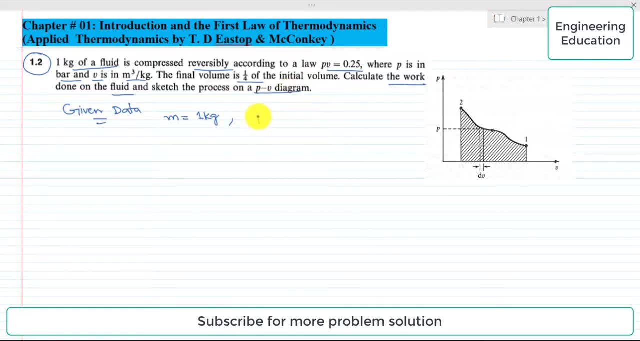 Reversible compression is: p-v is equal to 0.25 and the final volume is 1 by 4 of the initial volume. So v2 is equal to 1 by 4 of v1.. This is the given data and we are required to find the work done. 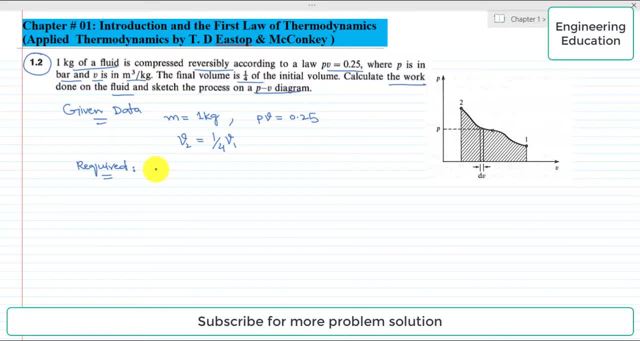 So only one thing is required in this problem, and that is work of compression. and then we have to sketch it on p-v diagram. So we will calculate the old solution of. So, before coming to the solution, Let us discuss the expression developed for the reversible compression process. 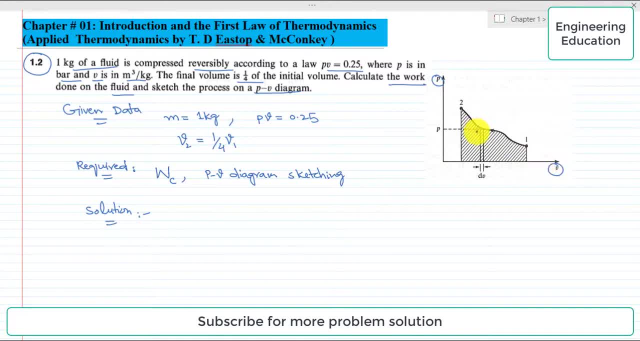 This is the pressure specific volume diagram. So now we know, Now we will calculate for the original. So we will calculate for the original. So we will calculate for the original, And it is the value of a single line. So now we will calculate for the two characters. pouvez? let me just give you the model. 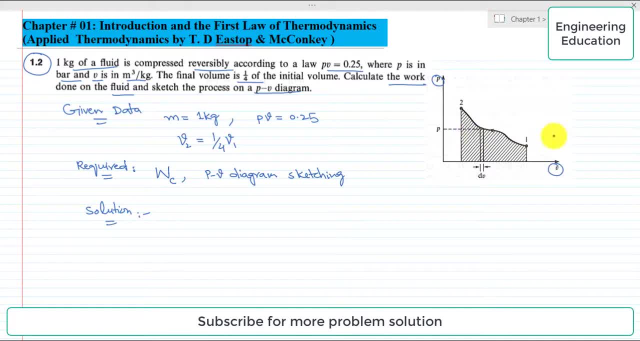 And it is the value of entity, And it is the value of entity. a general type of diagram, generic diagram. let's suppose this is state 1 and this is state 2. so from state 1 to state 2, looking to the direction of the. 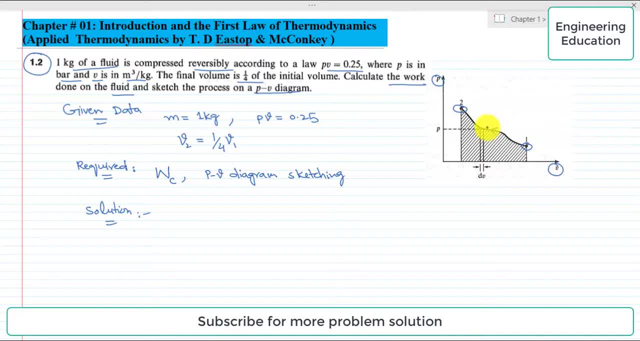 arrow. this arrow is from 1 to 2 and the expression developed for the general work done is: W is equal to minus M. integral P D V from the arrow. this arrow is from 1 to 2 and the expression developed for the general work done is: W is equal to minus M. integral P D V from. 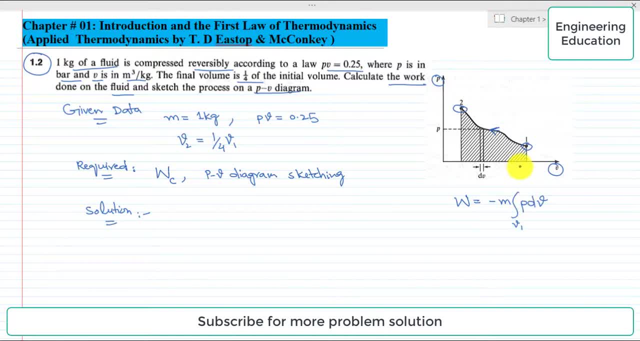 state 1 to state 2 means from V 1 to P 2, where V 1 is here and V 2 is here. so we will use this general expression in our solution. so W is equal to minus M limits from V 1 to V 2. 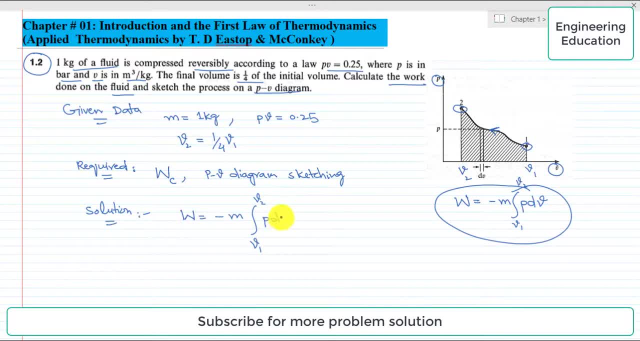 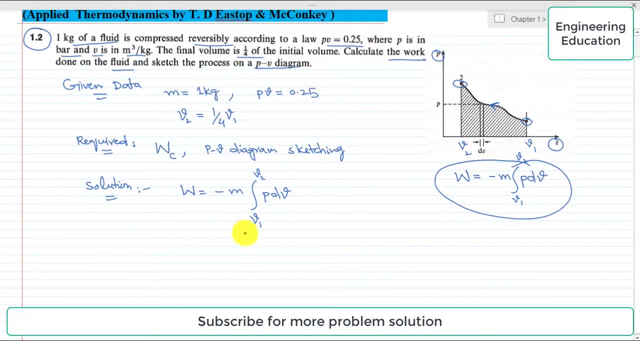 into P D V. here we know that P V is equal to 0.25. so, rearranging this, we can write that P V is equal to 0.25, so P will be equal to 0.25 by V. generally this is represented by C, so we can also write that P V is equal to C. C stands for: 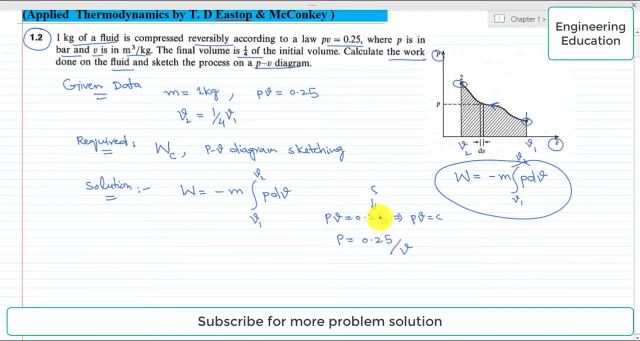 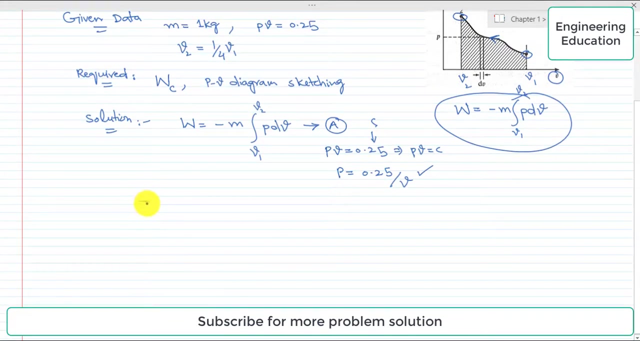 constant. in this specific case C is 0.25. so let's suppose this is equation A and so putting the expression P is equal to 0.25 by V in expression a, so we can write that W is equal to minus M limits from v1 to v2. P is 0.25 by P into dV, so 0.25 is constant. we can write that: 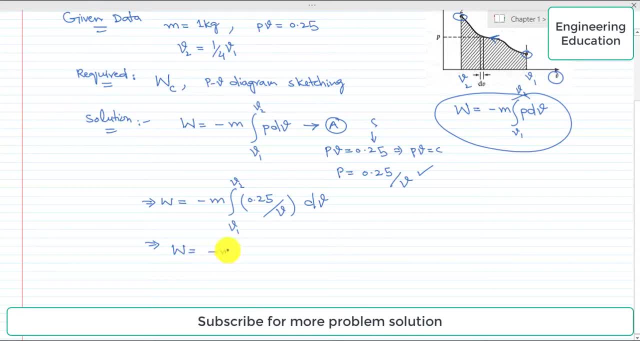 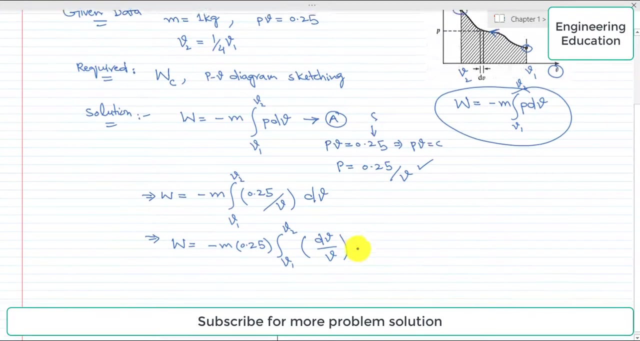 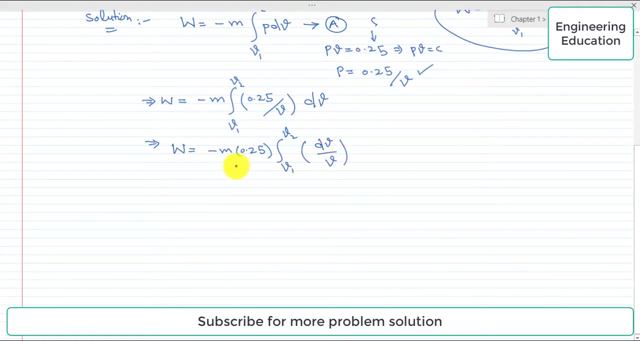 W is equal to田 M into 0.25 limits, v1 to v2, dv by V. so further, if we apply the integration and if we integrate it and put the value of M is equal to 1, kilogram is given in the problem. so W will be equal to minus 1 into 0.25 natural law of V from v1 to. 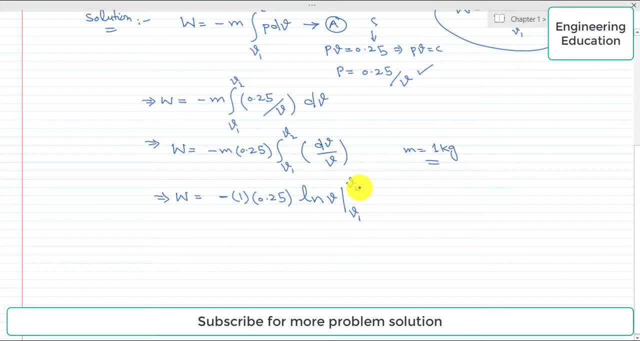 v2. so we're putting the limits in this. we can write there: minus 0.25 natural log of v2 minus natural log of v1. so we can also write this using Law of laws of log that W is equal to minus 0.25 natural. 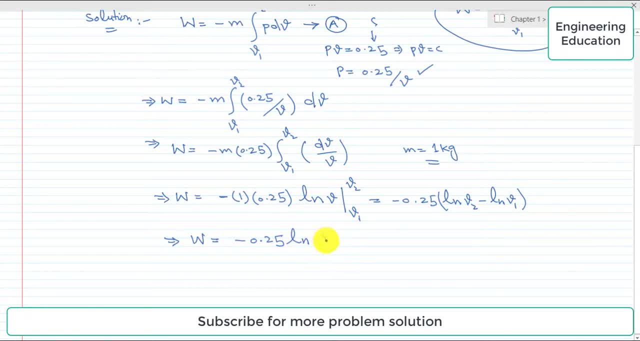 log of v2 by v1.. okay, End of question. Thank you. Further we have given that V2 is 1 by 4 times of V1, so we can write that natural log of 1 by 4, V1 by V1.. 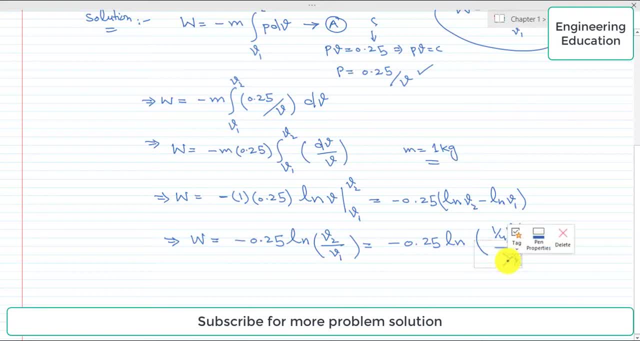 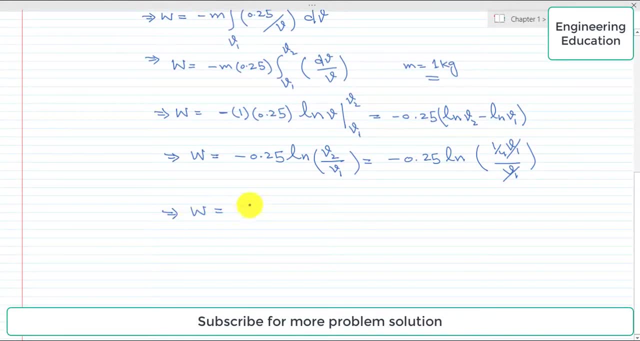 So this V1 will cancel with each other and we will get that W is equal to minus 0.25 natural log of 1 by 4 or 0.25.. So when we simplify this, the value of W comes out: 3, 4,, 5,, 6,, 7,, 8,, 9,, 10,, 11,, 12,, 13,, 14,. 15,, 16,, 15,, 16,, 17,, 18,, 19,, 20,, 21,, 22,, 23,, 24,, 25,, 26,, 27,, 28,, 29,, 30,, 31,, 32,, 33,, 34,. 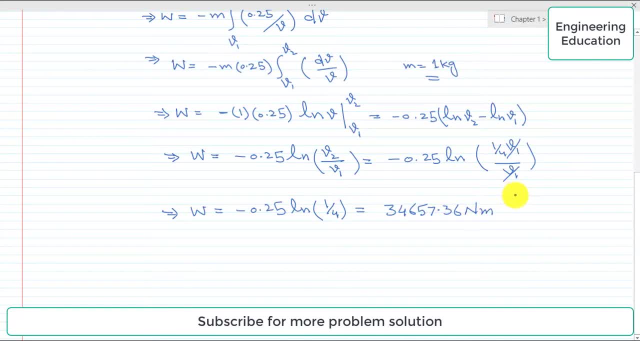 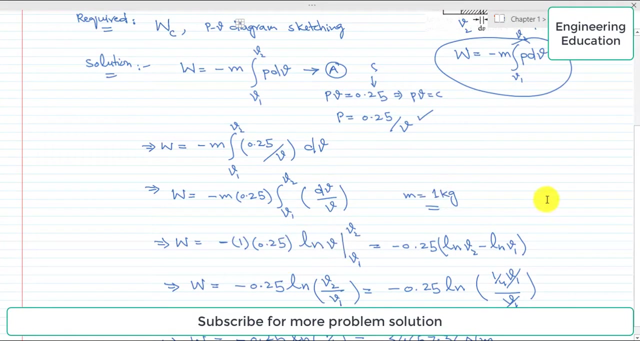 35,, 36,, 57,, 0.36 Newton meter. So this is the required work. Also, we have to draw the process, which is the compression process, on PV diagram. So for that we know about state 1 and state 2.. 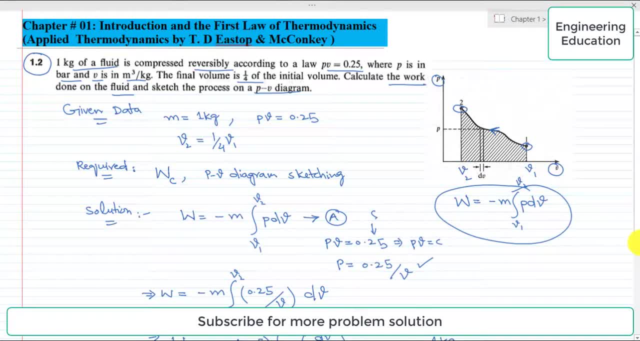 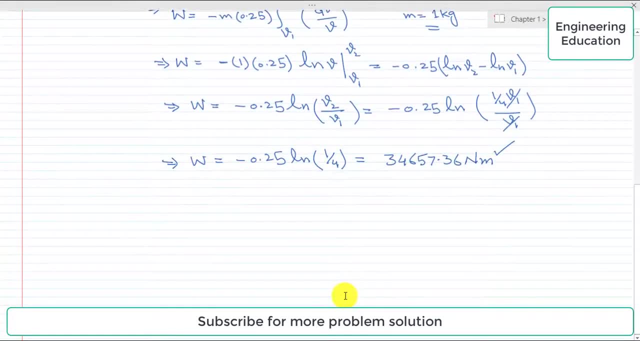 This is the general diagram and specifically we can draw the diagram for this problem as well. So the PV diagram for this problem will be PV. So this is the diagram: On y-axis we have pressure and on x-axis we have specific volume. This is P and this is V.